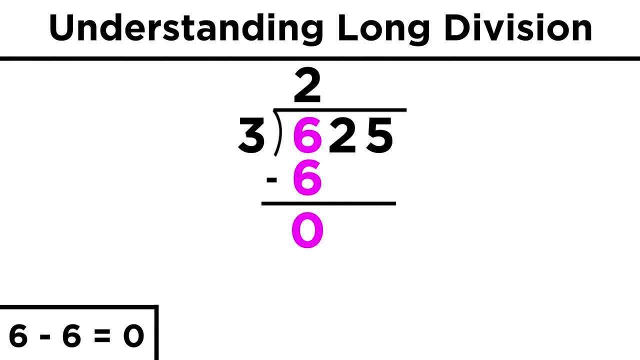 subtract Six minus six is zero. so we draw a line and write a zero here, Then we drop the next digit down and repeat the process. The next digit is a two. Three does not fit into two, or rather two divided by three is less than one. 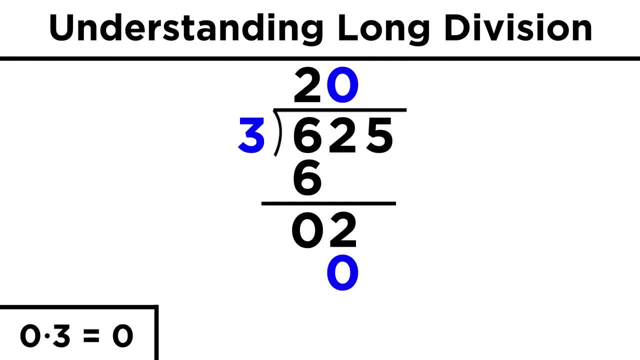 So let's put a zero here. Zero times three is zero. Two minus zero is two, and then we drop down the five. Three fits into twenty-five a little more than eight times, because three times eight is twenty-four Eight here. 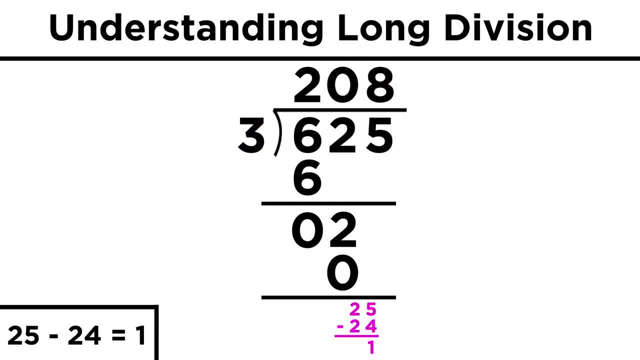 Then eight times three is twenty-four, as we said, and subtracting from twenty-five we get one. Now there are no more digits to drop down, and three doesn't fit into one, so this is called the remainder. Three fits into six hundred twenty-five, two hundred and eight times, with one left over. 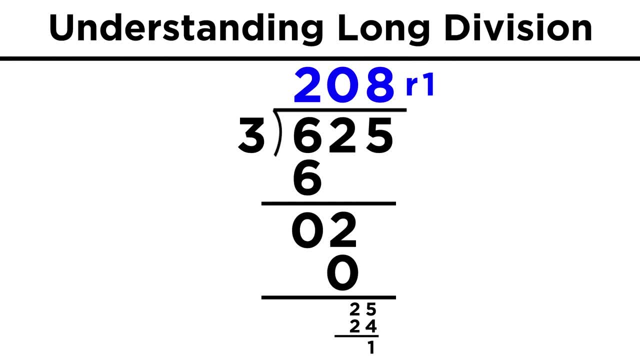 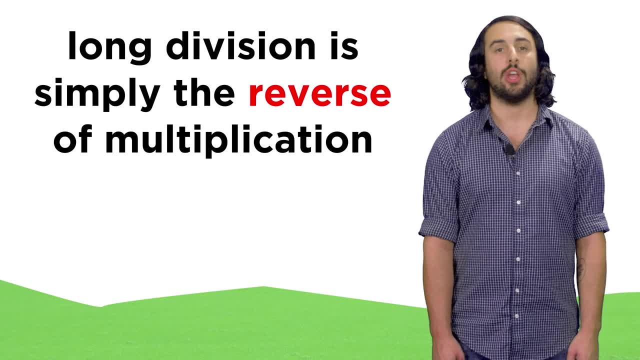 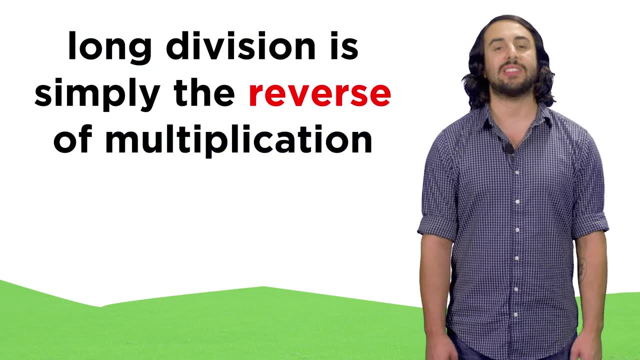 or we can say that six hundred twenty-five divided by three is two hundred eight, remainder one. So that's all there is to long division. We go one digit at a time, just like we did with multiplication, except we go left to right instead of right to left, since division is meant to be the reverse of multiplication. 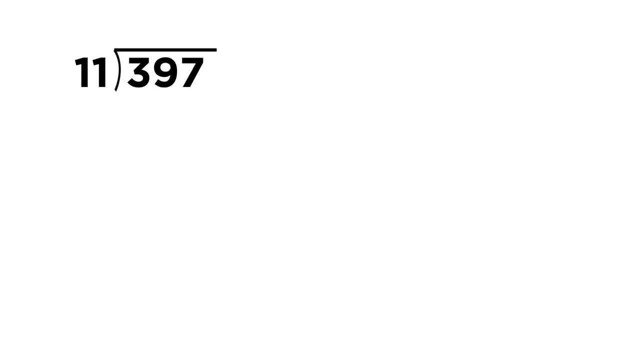 Let's try one more for practice. Three hundred ninety-seven divided by eleven. This time we have to divide by a two digit number. Eleven doesn't fit into three, so let's put a zero. get a zero down here, which leaves us with three. 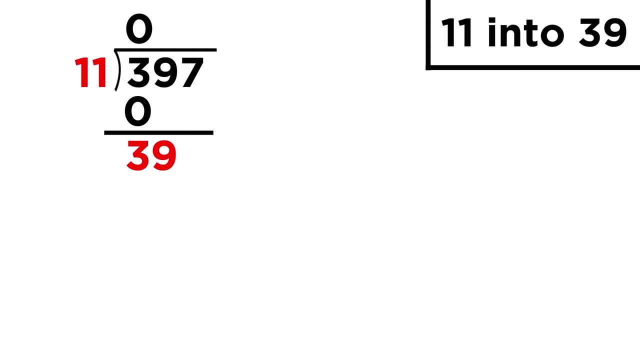 We bring down the nine Eleven does fit into thirty-nine three times. so we put a three multiply to get thirty-three, subtract to get six, and then pull down the seven Eleven fits into sixty-seven six times. so we put a six multiply to get sixty-six. 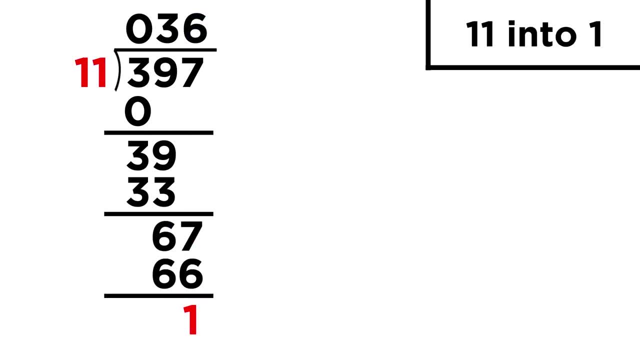 and subtract to get one. Eleven doesn't fit into one and we've run out of digits in the dividend, so that will be thirty-six, with a remainder of one. Okay, In order to avoid any more dangers, we could keep going to get decimal places. 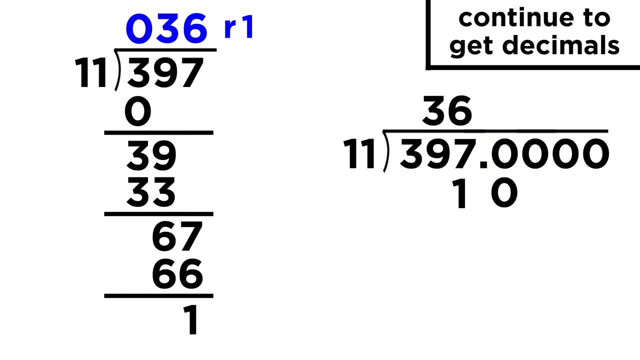 Just put a decimal here and add a zero, Drop it down to get ten. Eleven doesn't fit in ten, so we put a zero, multiply to get zero and subtract to get ten. Then we pull down another zero and we get one hundred.